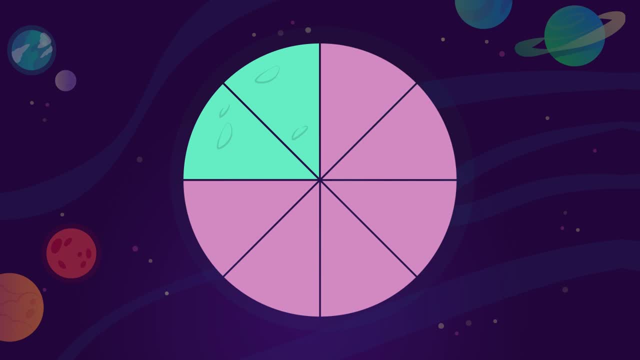 they grow apple trees and lemon trees. If four of the eight fields are planted with lemon trees, how many fields are planted with apple trees? To find out, we'll have to subtract fractions. We need to subtract the total number of fields planted with fruit trees from the number of 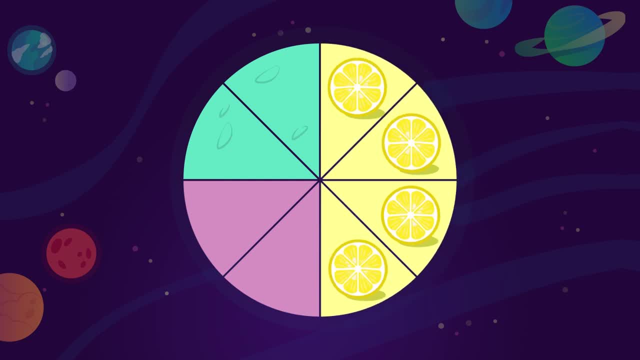 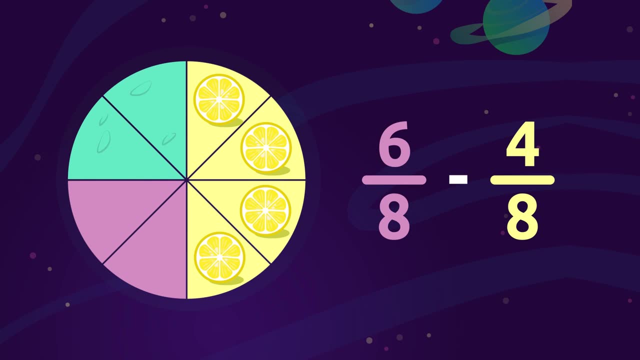 fields planted with lemon trees to find out how many apple tree fields there are, meaning six-eighths minus four-eighths. Do you remember how to do this math operation? Remember that we should put the same denominator in our answer, In this case number eight. 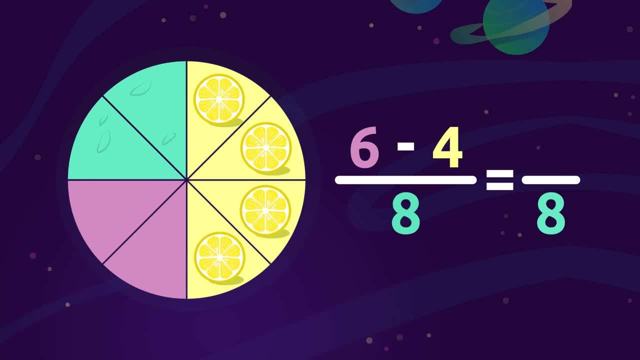 Now, to calculate the number of fields planted with fruit trees, we need to subtract the total. we subtract the numerator six minus four, which equals two. The result is that two of the eight fields are planted with apple trees. That is two-eighths. Will you help me figure out something? 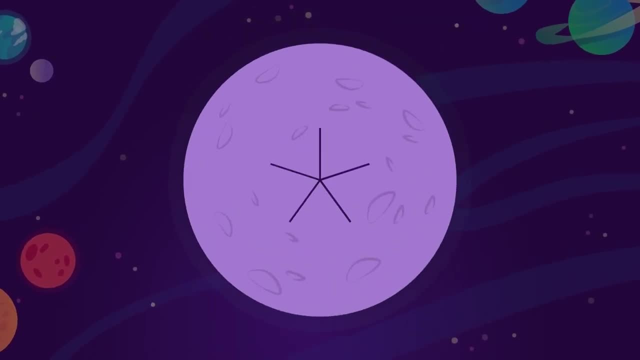 else. Planet LearnTurn is divided into five equal parts. On this planet there are wooded areas and areas with houses. We need to find out how many areas are planted with apples On this planet. there are houses. If they built houses on three of LearnTurn's fields, how many parts of the planet? 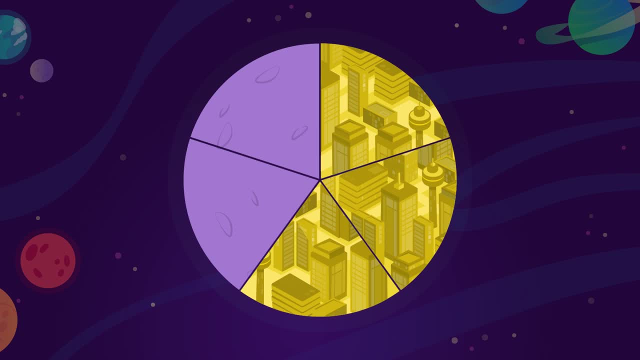 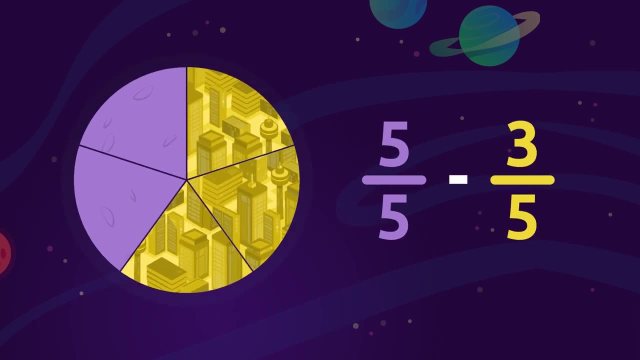 are covered with woods. To find the solution, we'll need to subtract the fractions Five-fifths minus three-fifths To work out the answer. first we leave the same denominator- In this case it's number five- And then we subtract the numerators, In this case five minus. 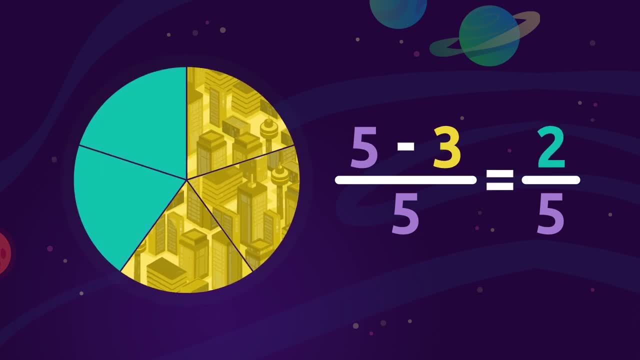 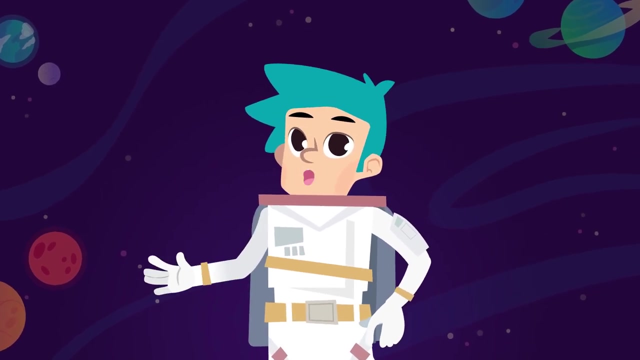 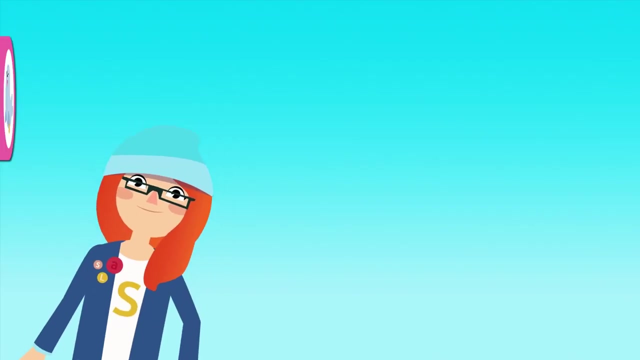 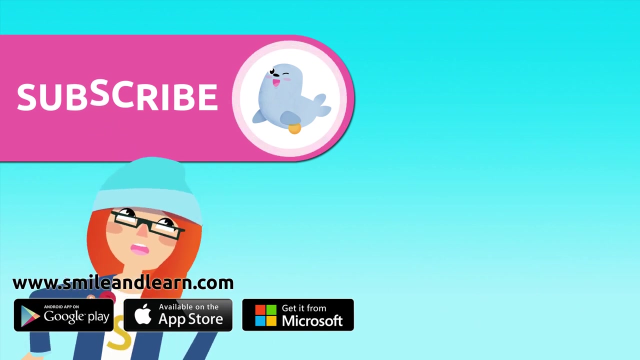 three, which equals two. The result is that two parts of LearnTurn planet are covered with woods, That is to say two-fifths. Congratulations, Now you know how to subtract fractions with the same denominator. See you around. Subscribe by clicking on the seal Ah, and if you want to keep watching more videos, click on the boxes.